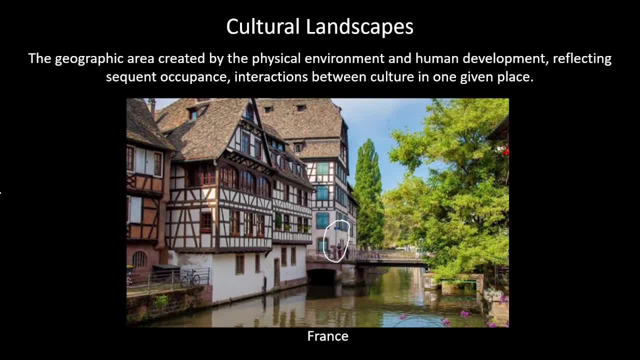 They've kind of worked with it building bridges over the water instead of just building on the water and like moving it or something, because that's what they're doing. Technology is great nowadays, So it shows kind of what they do, how they work with the environment. 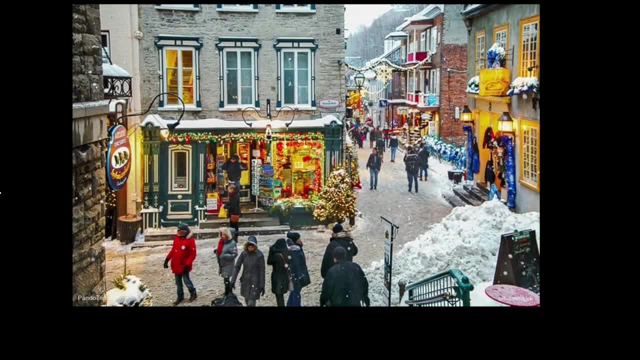 All right, here is another place. No, it is not France. Can you guess what it is? And we'll just go through this as we go on. So let's look at some places, so not places. elements of the culture. 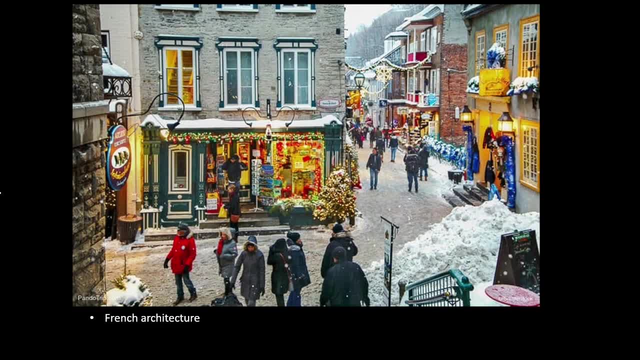 So we see French architecture, So I said it's not France because of the similar French architecture in this place The buildings are kind of crowded together But there is snow, so it's not going to be a place like Florida, Florida. 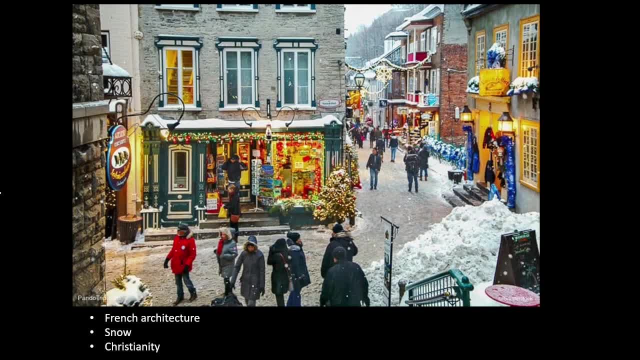 It's been snowed here since like 89, I think. Christianity is represented through the Christmas decorations, and that is a Christian holiday, So Christianity is probably a prominent religion in this place. There's both men and women in this picture. 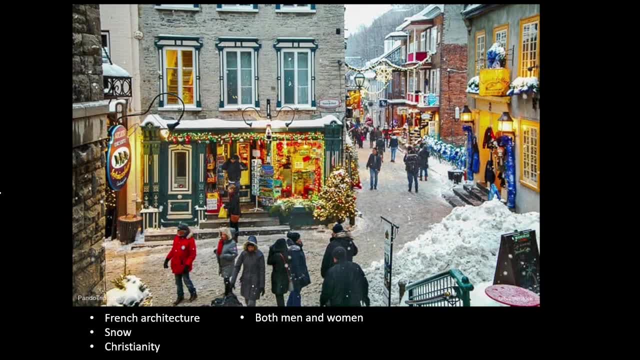 It might be a little blurry, but there is men and women, So women aren't forbidden to go outside or something. But there's a lot of people outside. It's not really a big like war problem. I guess There's no cars, but a little snow and trash can on the side of the house. 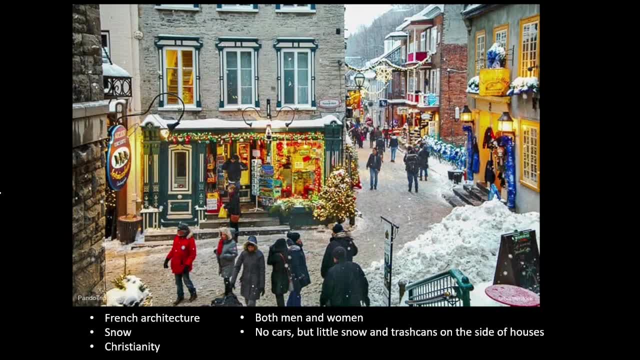 So vehicles have gone by. We see these trash cans. I'll circle them for you. There's one, There's one right here as well, But those are trash cans, So maybe they have, like a garbage man come by and take out their trash. 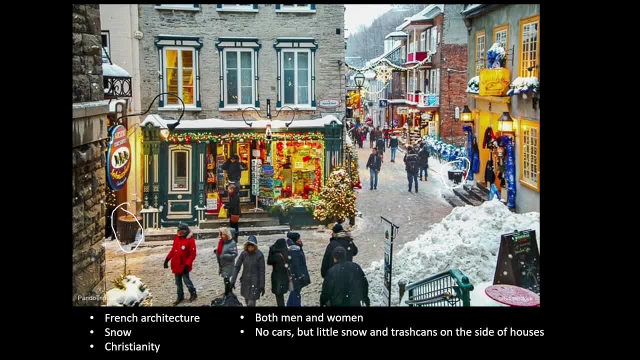 So that's what things look like, And what place do you think this is, Or what region do you think this is? Well, this is Quebec, Canada, So it's going to be on the eastern side of Canada, And there's a lot of French characteristics here. 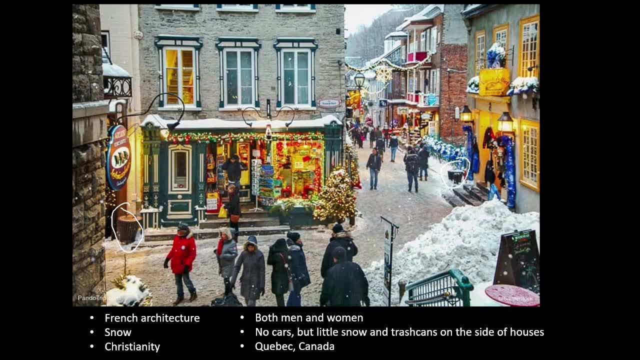 So there's some English and French Actually on the signs And the reason for this is because of previous French colonization on the eastern side of Canada, where Quebec is, So we see a lot of French culture there through the relocation diffusion. 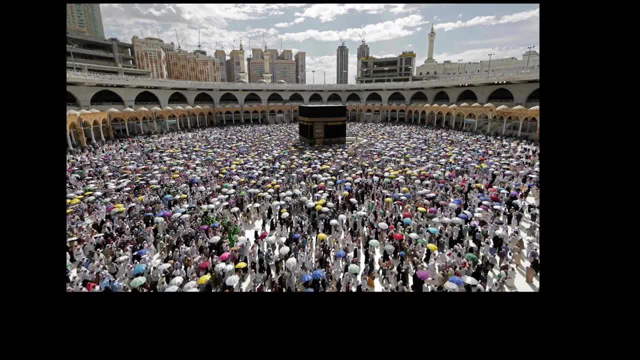 Really, really cool. So yeah, We just analyzed the cultural landscape. Let's do another one. This one is not Quebec, Canada, So let's look through this. You probably know what it is, just based off looking at it. 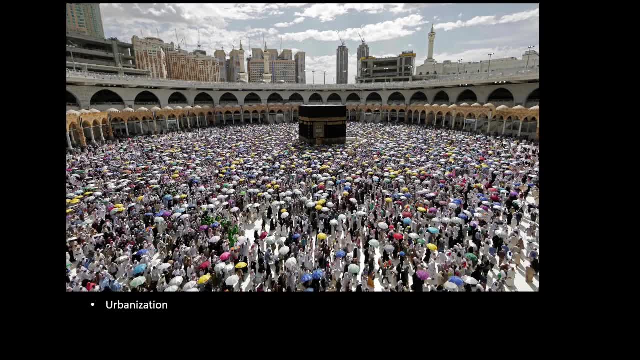 But if you don't, that's okay, We'll continue going on without it. So we see an urban area And we see actually like cranes and stuff on these buildings. So it's definitely Urbanizing still. 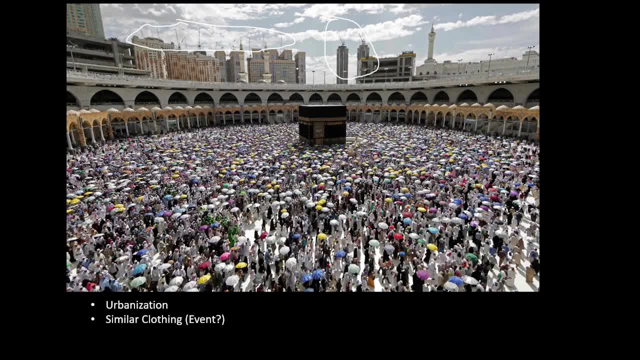 It's not like completely developed. There's similar clothing So they might be at an event And it looks kind of religious, So it might be a religious event. And this is actually the Hajj, where people go to this place for Islam. 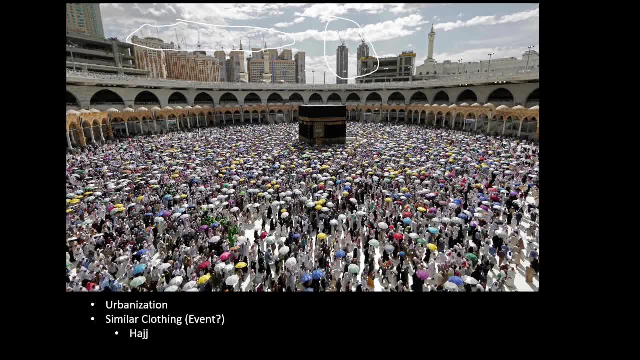 Because it's part of their, like pillars. I think I'm not Islamic, So I don't know anything about it. And there's hot weather And this could be reflected by the umbrellas we can see in the sky that it looks kind of hot as well. 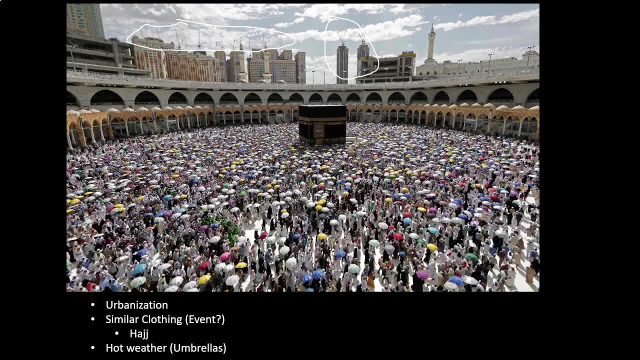 It looks, Um, Not cold. We don't see snow or like ice and stuff, So it looks pretty hot. It might be a mild temperature, Maybe in the 70s. There's a cluster of people, So the cluster of people, could you know, signify about the events? 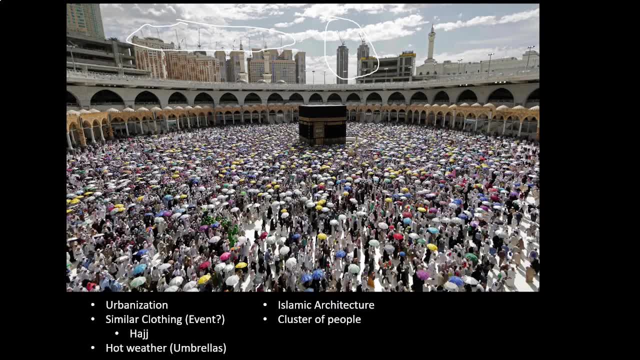 Or there's a lot of people there. There's Islamic architecture as well, So I could like circle that. This is Islamic architecture right here, So that's reflecting Islam. And this is Mecca, Saudi Arabia, where people go on the Hajj. 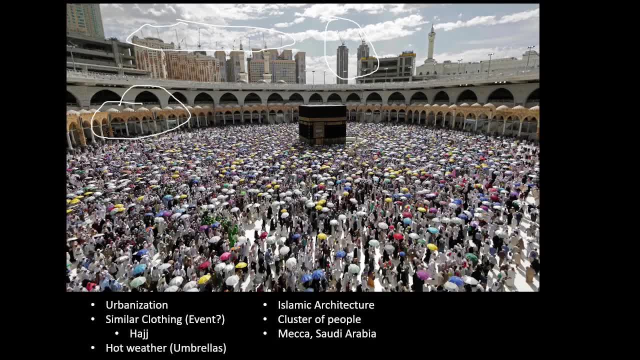 So we can use that to kind of pinpoint our region. Islam is kind of popular. People are in the Middle East. That's where it's hearth is, Saudi Arabia Kind of explains why Mecca is important. This is a shrine right here. 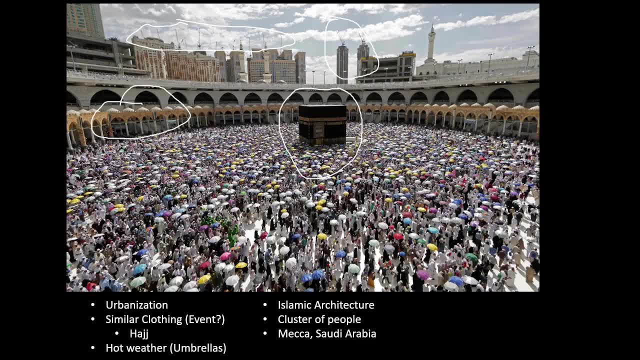 And there are pillars of Islam. They have to go to the Hajj, to Mecca, at least at some point in their lives. All right, Here's another thought. You probably know what this is as well, if I'm looking at it. 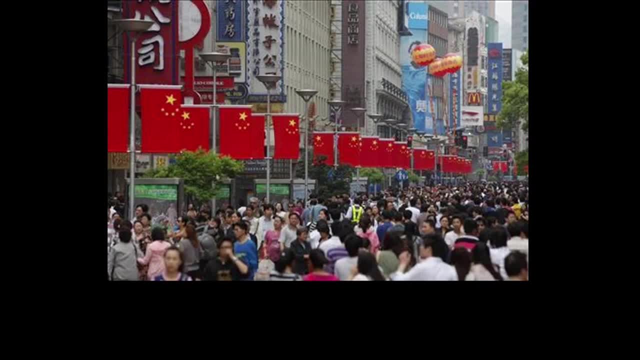 But if not, that's totally fine. We'll go through some elements of it. So we see the Chinese ethnicity in the pictures, Or just some Asian ethnicity in general as well. We see Chinese, Chinese culture, So we can see the language. 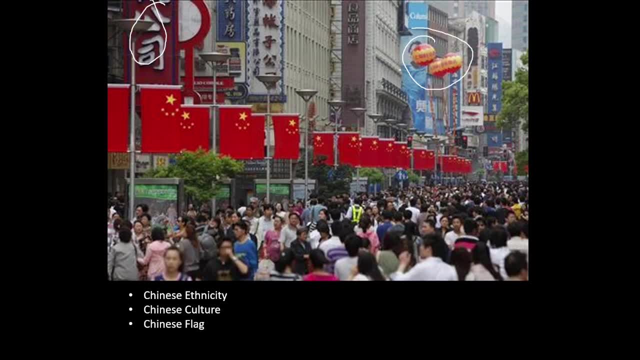 We see these lanterns here, That is Chinese culture, The flag as well, That's the China flag. Then we see globalization. So I see a McDonald's here in the background. So we see businesses kind of going international, International. 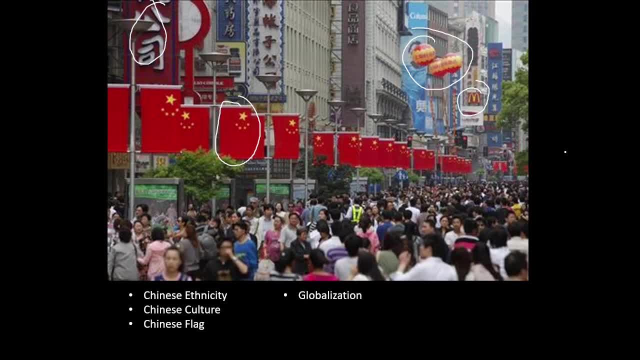 International, Going through various cultures and impacting various societies and places. It is urbanized- We can definitely see that from all the buildings in the image- So it's very crowded. So it's probably developed As we move up the city. 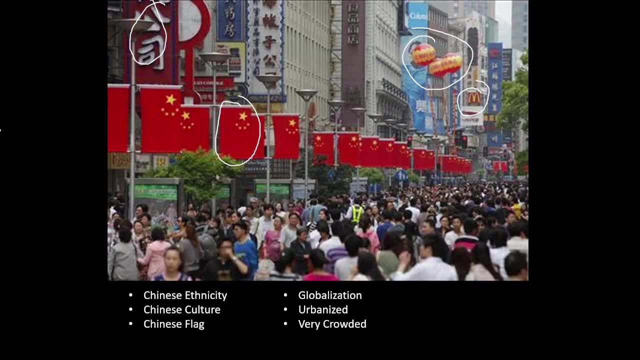 We can see the stages of the demographic transition model, Unit 2.. We see a higher population, as we see here in this very Chinese society, And of course we see urbanization take place as well, Which leads to a decrease in population growth. 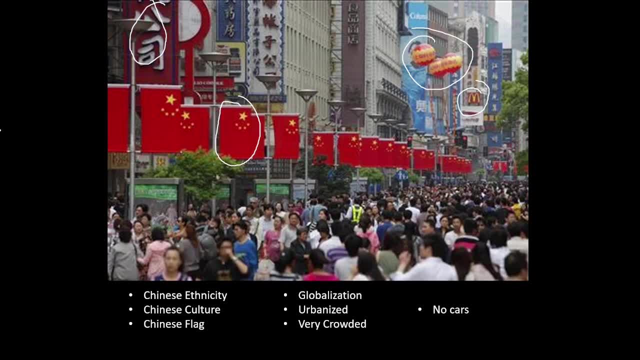 Career birth rate. There's no cars as well. No cars, Which could mean that there's not room for cars. People can't maybe afford the cars, Or it's just not part of the culture in general, And this is, in fact, China. 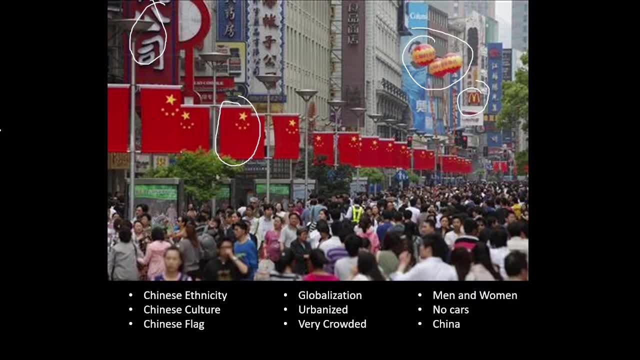 We can piece that together by the culture, And then I don't know why these are showing up later than they are. They shouldn't be doing this. But there is men and women. Now, one thing I do want to point out is that you can't always determine gender roles from a photo. 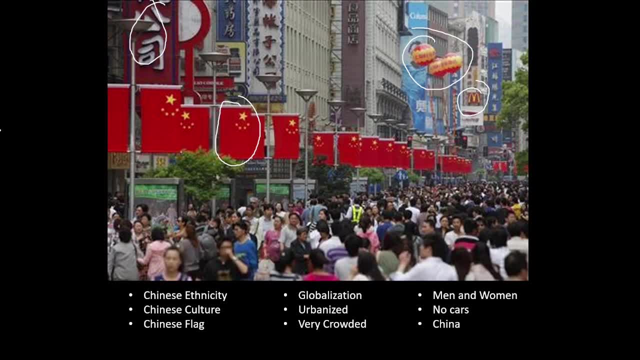 And most of the time you cannot do that. So if you look at a photo and you see just men, that can't conclude that men are dominant in the country Or they have gender roles. And we see a picture of China and there's just men in the image. 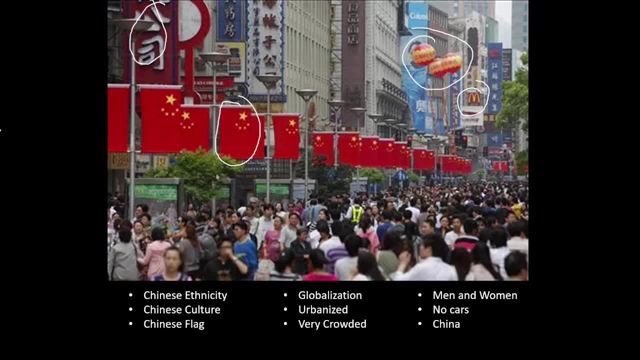 We can't conclude that this place in China is still adapted to Confucian standpoints, Where women are more dominant, Where women are inferior to men. I think that's how you say it. I might be wrong. So we can't conclude that just from an image. 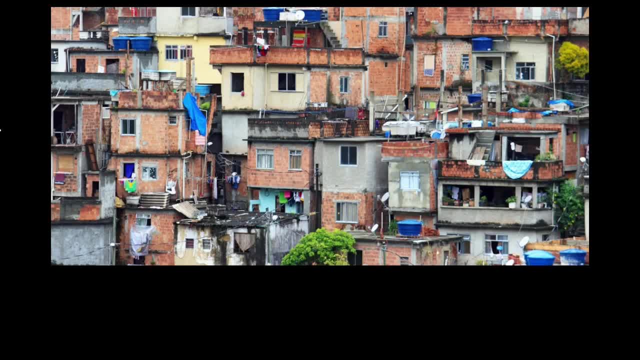 Alright, here's the next one. If you know this place as well, that's great. we'll go through it as well. So it's a very crowded environment, So there might be a high population. There's lots of trash. 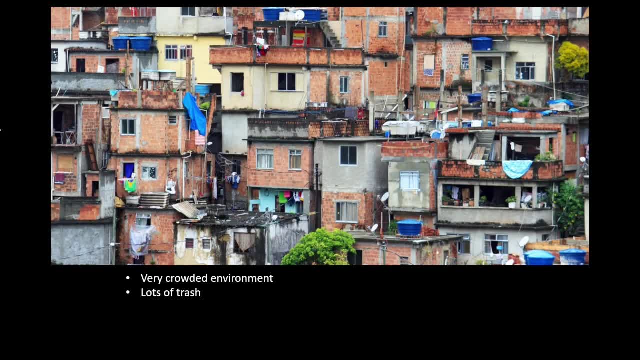 So it's not really clean, People don't really care about it, But it's not really developed as well. So, yeah, But it is urbanized. We do see buildings. We see the clusters of people together. There's Hispanic architecture. 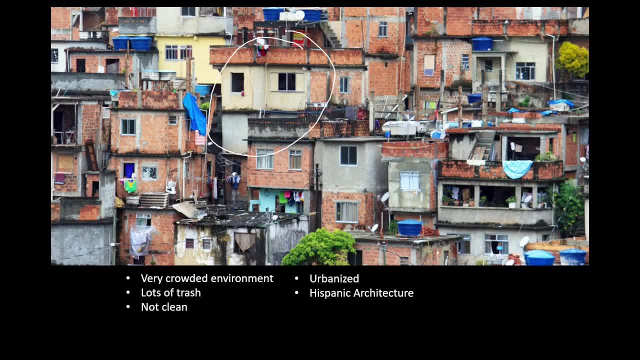 So this kind of style of buildings It's pretty Hispanic, So it might be in Latin America. There's technology, So there's satellite dishes, There's wires and stuff, So they do have some form of technology, And this is Brazil. 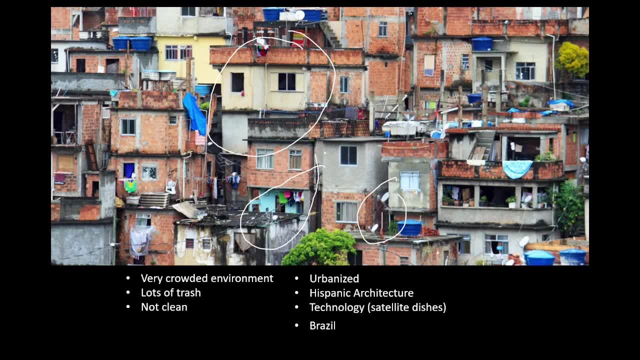 These are the favelas in Brazil, also known as squatter settlements. You'll learn more about this in Unit 6.. And these are kind of cool because they're very clustered areas. Squatter settlements develop because urbanization happens so quickly that there's not enough space for the people in the urban city. 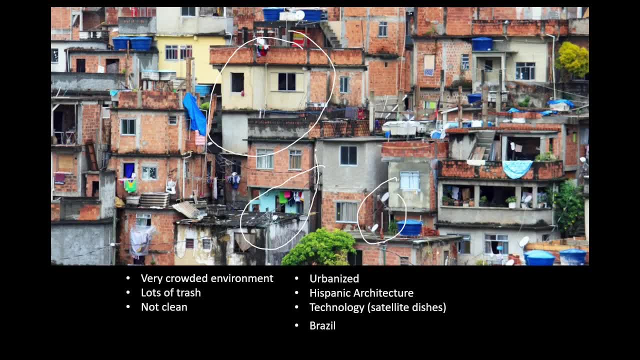 That's why they're called squatter settlements. It's also affordable. So they kind of build these illegal settlements called squatter settlements And they have some of the cultural elements and technology, But it's very crowded. There's lots of trash. 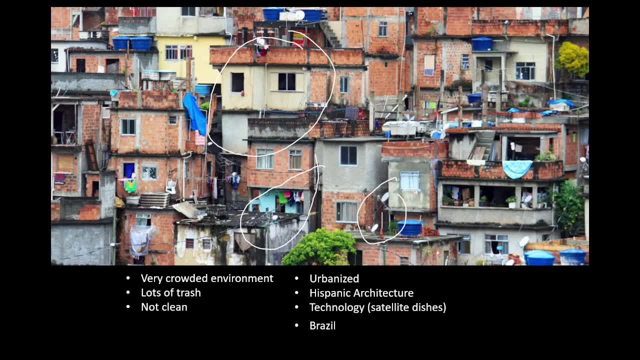 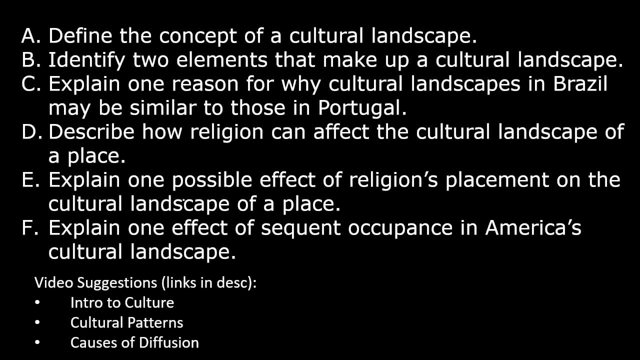 It's not clean, There's high risk for disease and all that. All right, And that's the end of the video. We just analyzed some cultural landscapes And that's about it. So I want you guys to do the FRQ on the screen using what you've just learned. 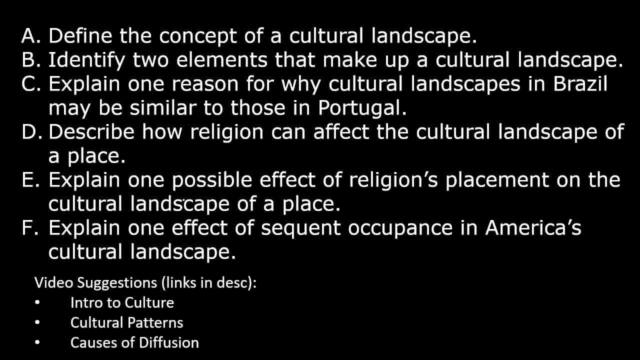 Some suggestions for people who want to watch this. Please like and subscribe. It is free. It really does help me out and motivates me to do more videos. So, yeah, You guys can watch the next video, which is on cultural patterns.